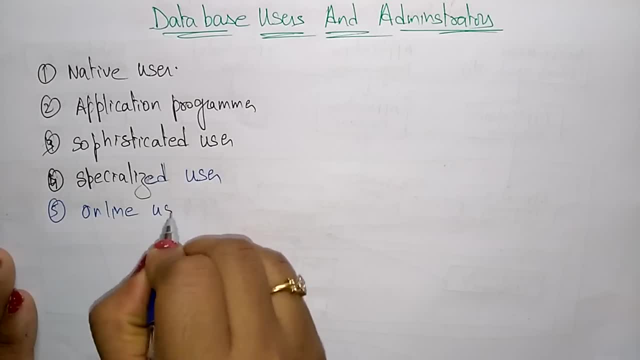 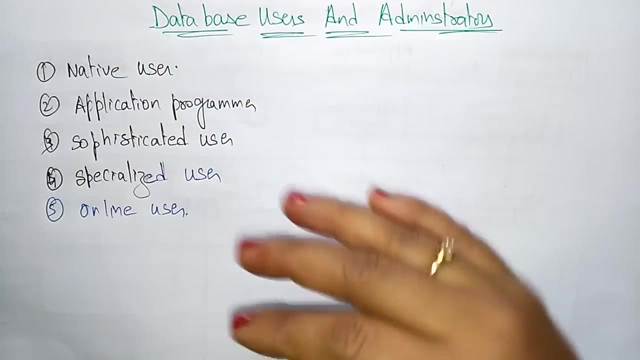 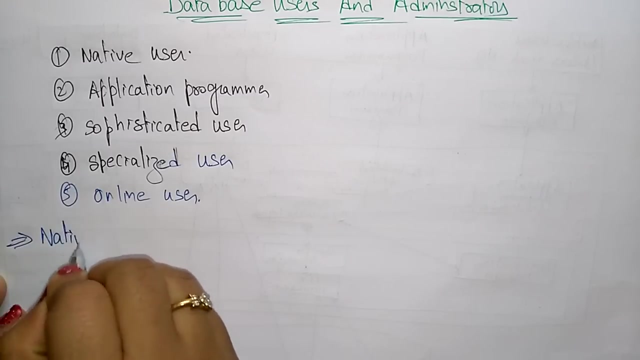 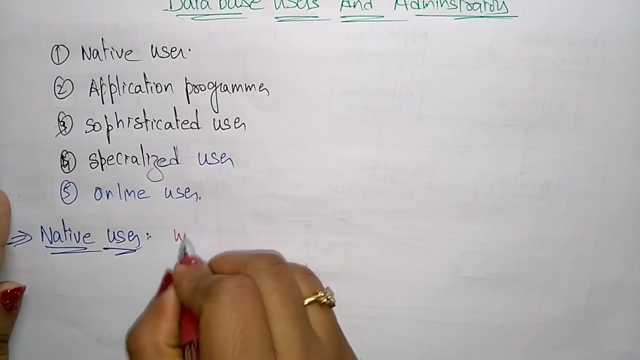 and next is online user. so these are the- uh five users. you call it as a database user means the. these people are accessing the database. now let us see one by one. so who are native users native users? so native users are those who need not be aware of. 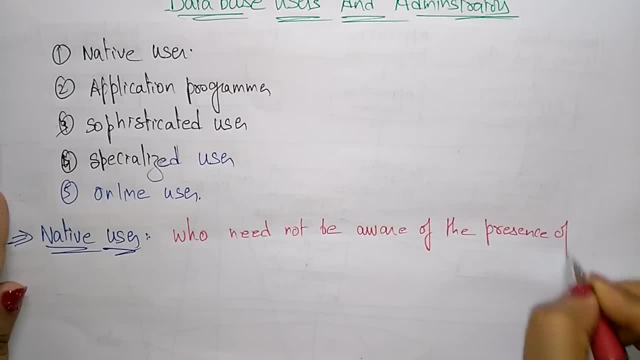 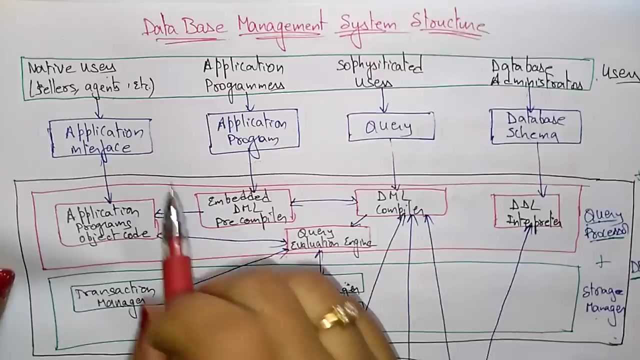 aware of the presence of database system, so they don't know about the presence of database system. they are just accessing the application, whatever they are using that, so they need not be aware of the presence of the database system. so in the structure i had said, native users are nothing. 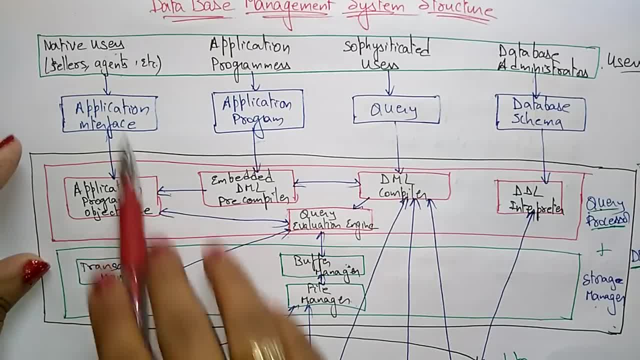 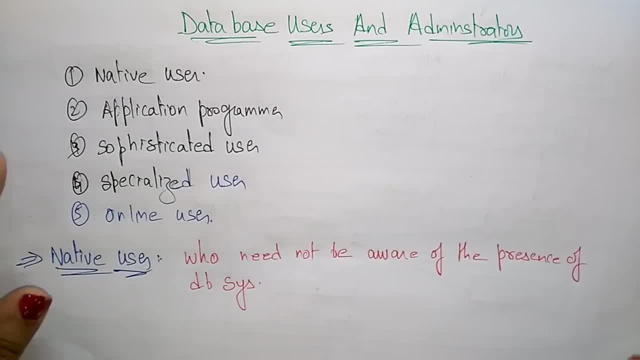 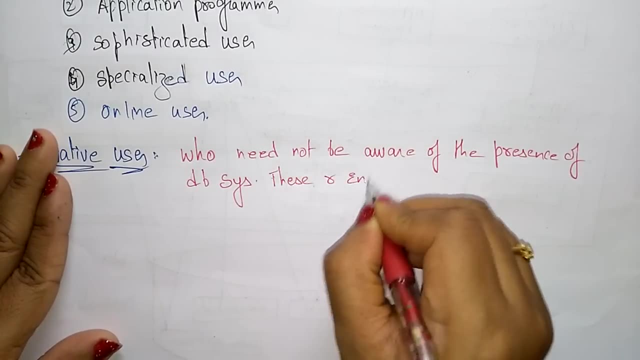 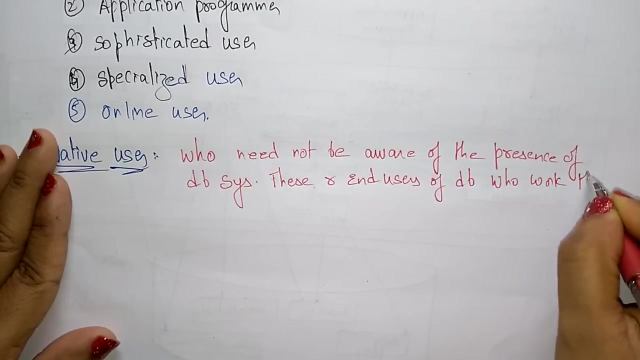 but the sellers and the agents, so they will interact with the database only with the help of the application interface, so they are not aware of the presence of the database systems. okay, and these are the you can also call. these are end users of database who work through menu driven applications only with 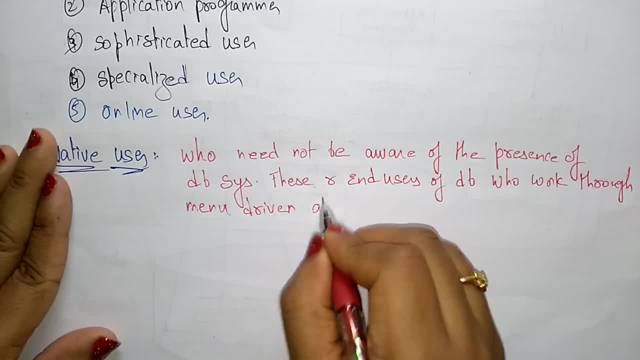 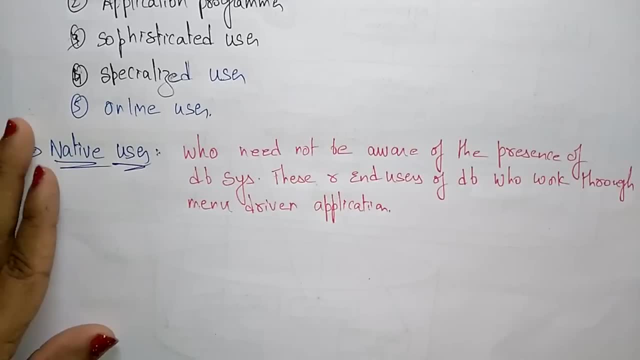 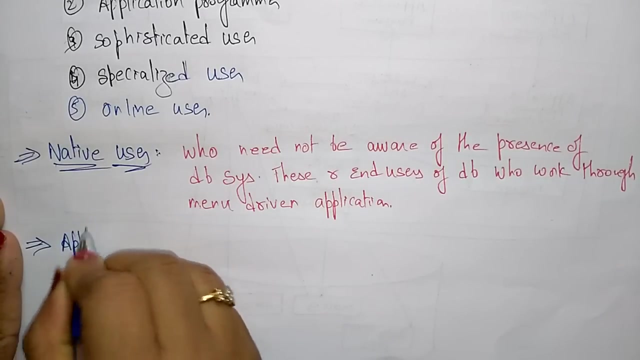 the application. whatever they are seeing on the screen, just with the application they are interacting with the database, so they don't know what type of database system is present inside those. you call it as a native users. now coming to the next. next is a application programmer. so, application programmer. 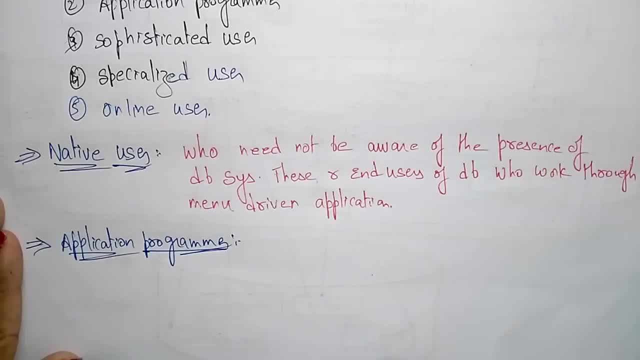 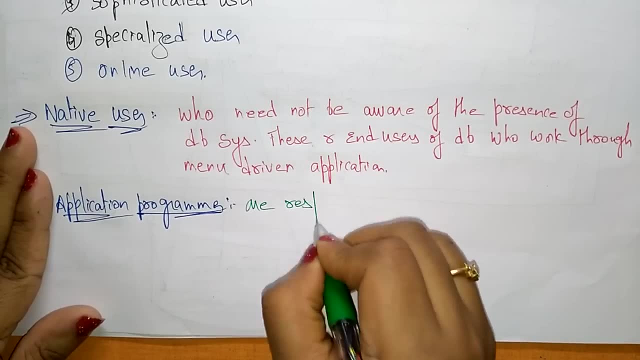 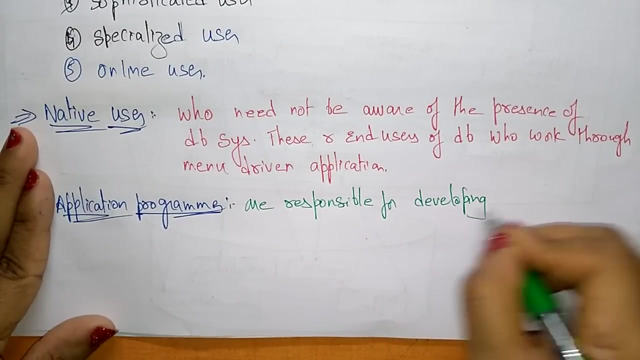 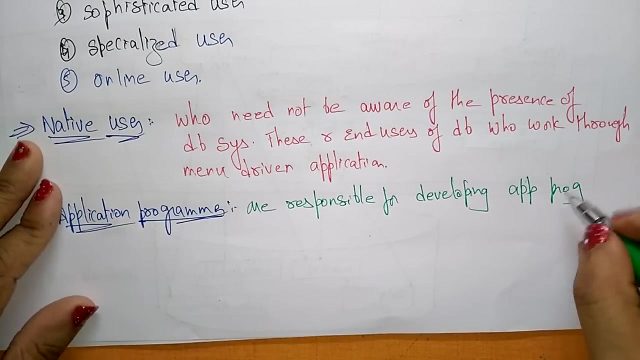 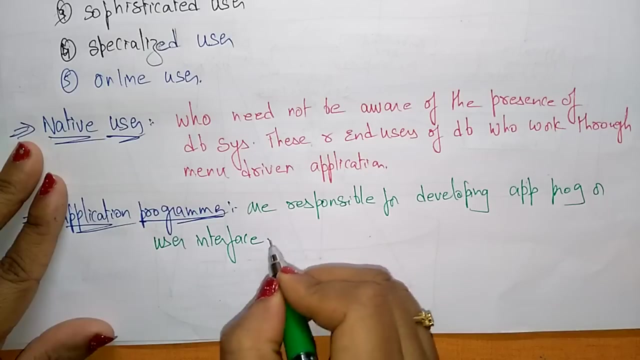 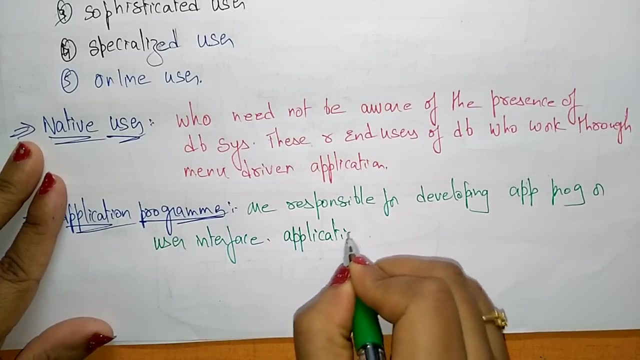 is a person who develops the application, he can interact with the database. so the application programmer. or responsible for developing application programs, so he is the main responsible for developing the application programs. or user interfaces. user interface, so here the application program will be written. so always the application program, whatever it is, the different application programs, if you are taken. 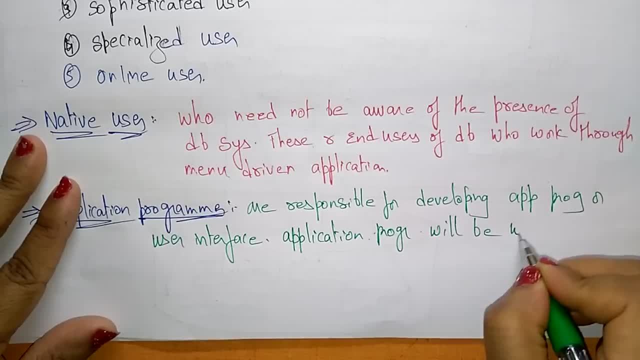 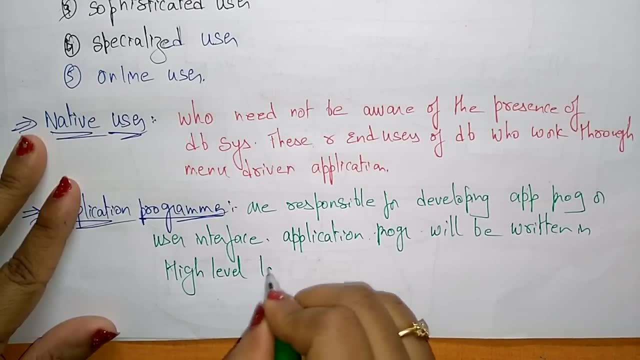 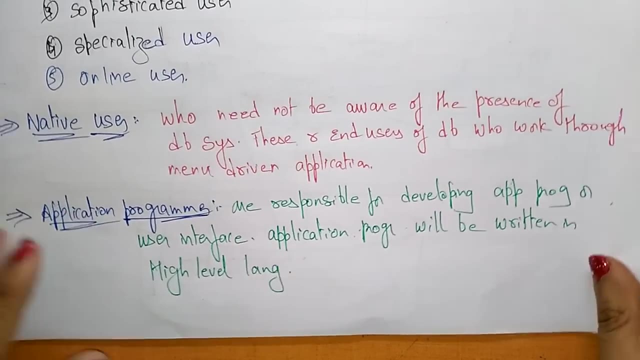 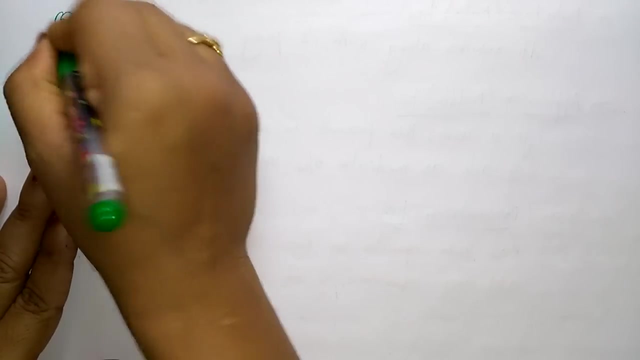 will be written in high level language. so examples, or C, C++, Java, those are all written in the high level language by the programmer. so those you call it as application programs. now, the next is the sophisticated user. the third one is who you call it as a sophisticated user, the user. 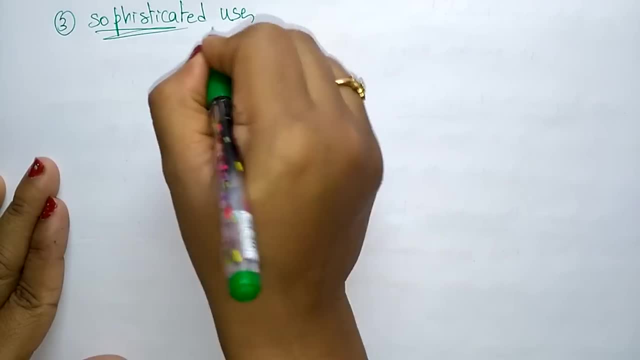 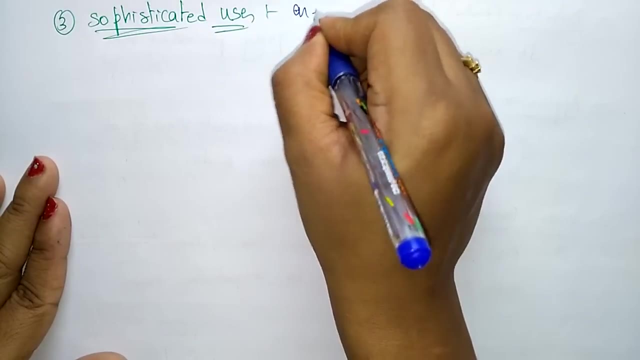 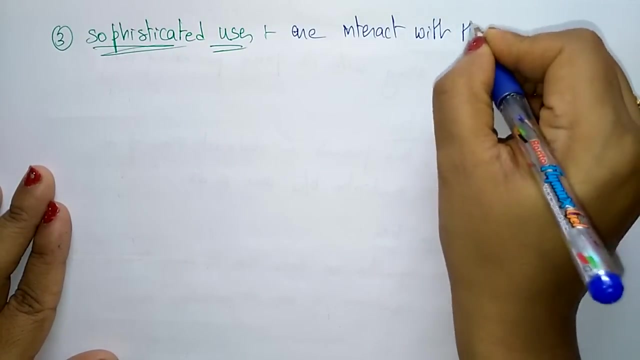 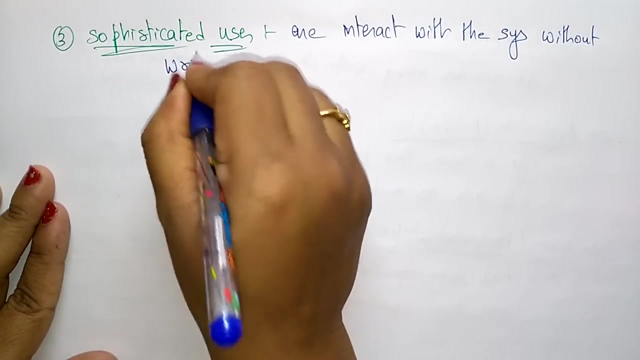 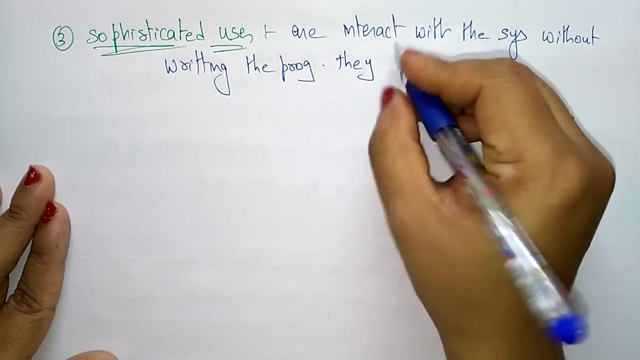 who interacting with the database, only with the queries. those are the sophisticated users. so let me write sophisticated users or interact. interact with the system without writing programs, without writing the programs. they are not writing the programs to interact with the database they request only with the help of the query. 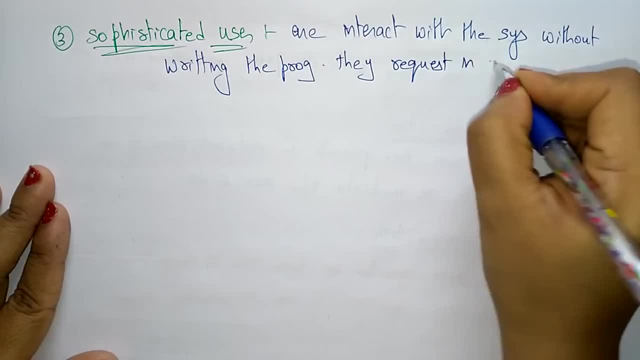 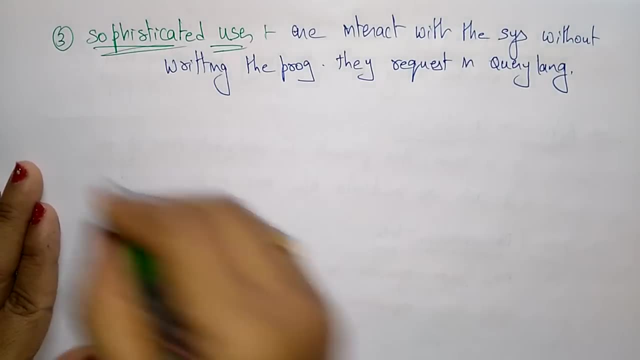 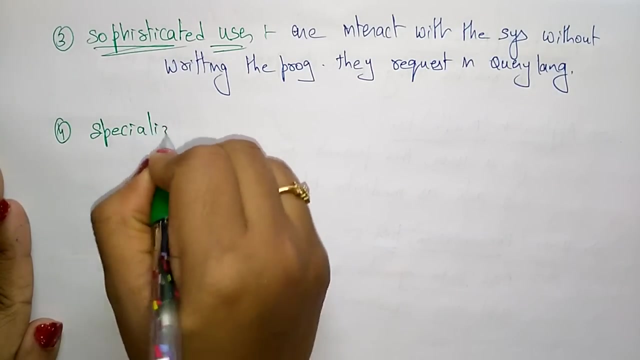 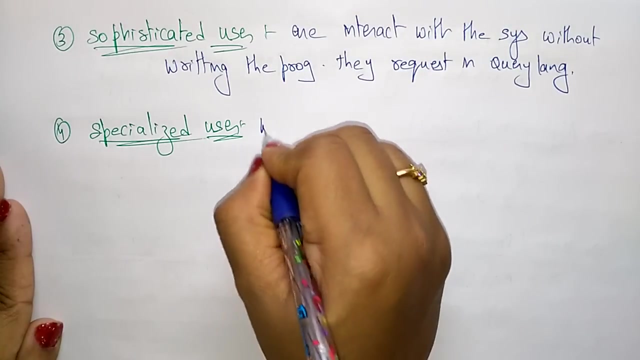 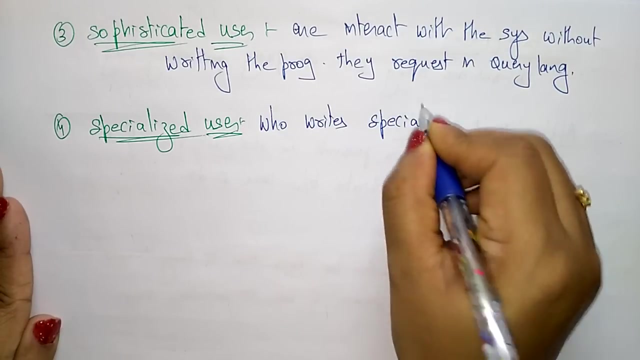 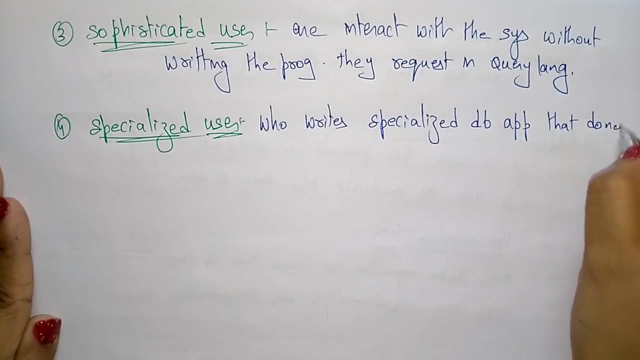 they request inquiry language, so they won't write the program to interact with the database. and the next fourth one. fourth one is a specialized user. so specialized user means who writes, who writes specialized database applications that do not fit, they won't fit, that do not fit into fractional database. 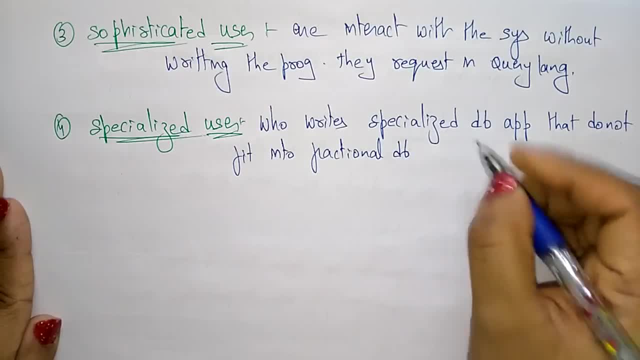 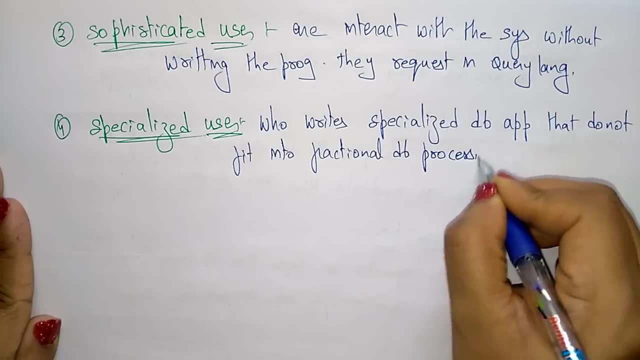 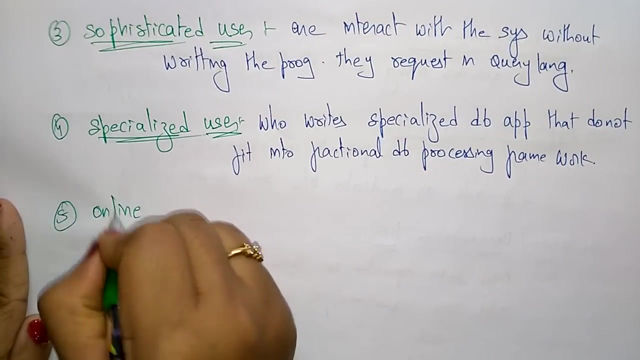 so those you call it as a specialized user, that do not fit into fractional database processing framework, so those you call it as a specialized user. and the next one is the online user. the last one database user is the online user. so here the online users who may. 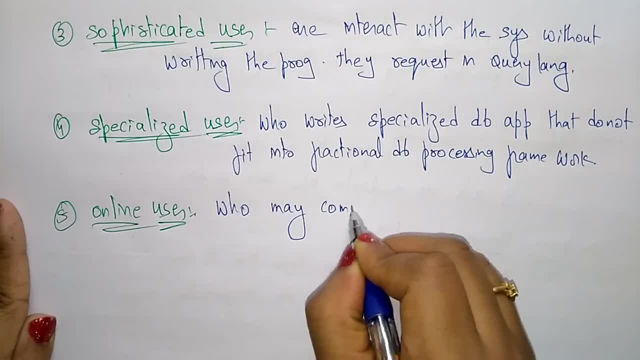 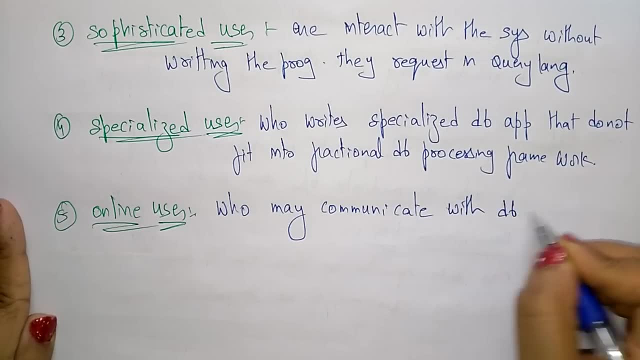 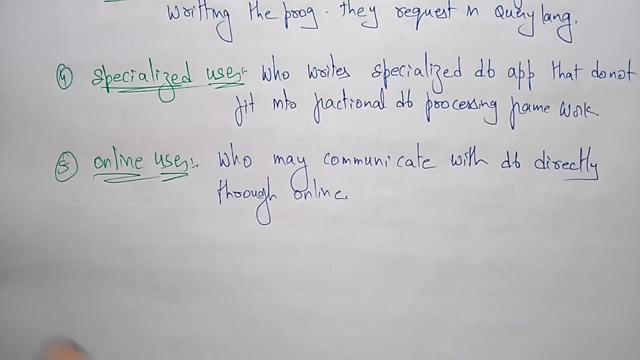 communicate with database directly through online. so the person who communicate with database directly through online- those you call it as an online user- so these are the different users that are present in the database- means they are accessing the database, so those are call as database users: native users, application programmers.